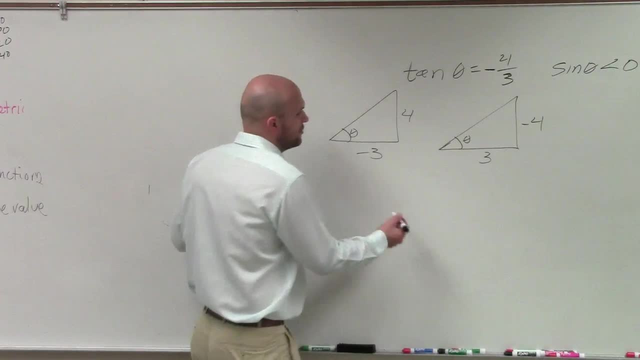 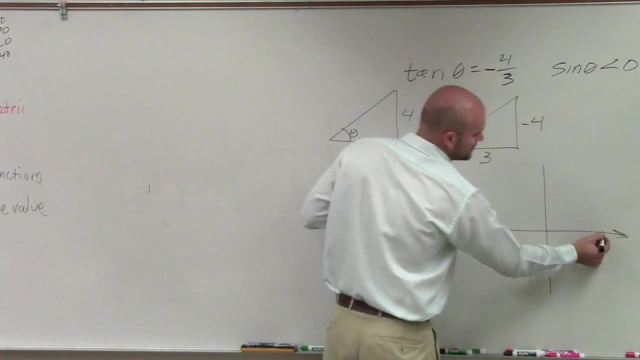 The reason why, Justin, is because what I want. what I want to do is: let's go and write them on a Cartesian coordinate. If my opposite side was negative, that means I'm going to go down negative 4, right? So it looks something like this: 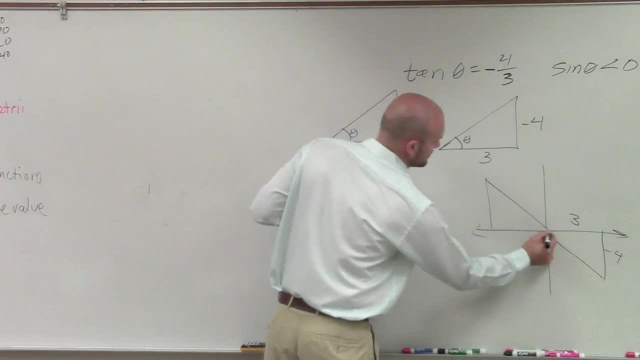 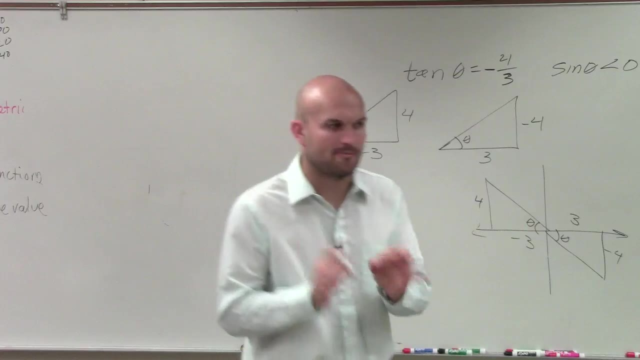 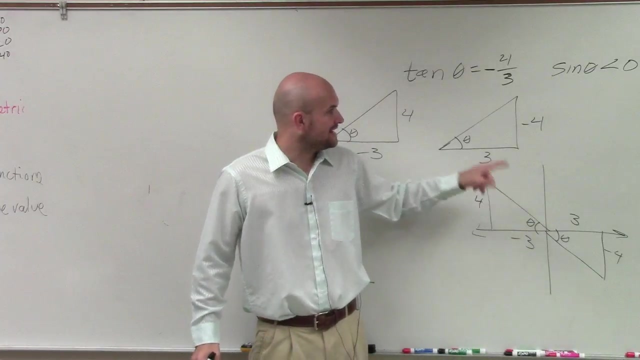 Or if my 3 was negative, it looks something like this: Remember, I'm always going to have my theta in my central angle about my origin. okay, That's never going to change, But those are my two possible triangles. So those two possible triangles produce a tangent of theta which is negative: 4 over 3.. 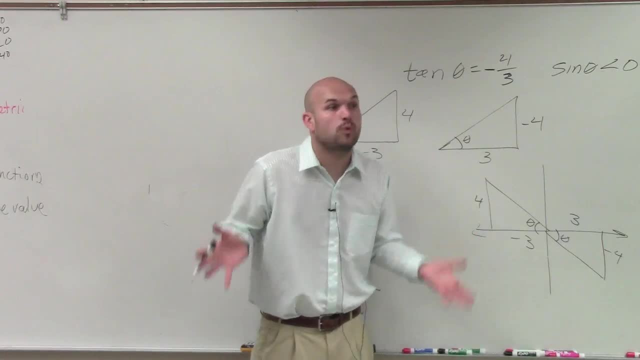 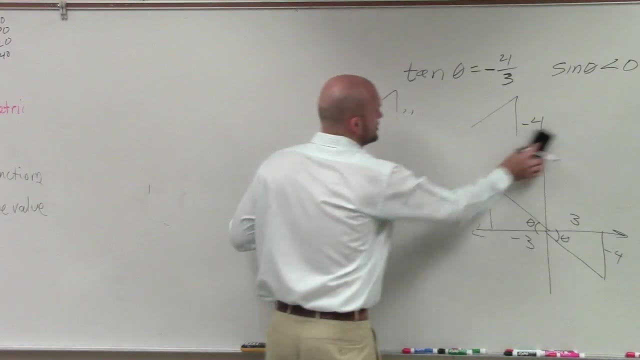 Does everybody agree, Okay? So therefore, I'd have to do this problem twice to provide both answers. We don't want to do that, though, right? Okay, we only want to do this once. So what we have is we have a constraint. 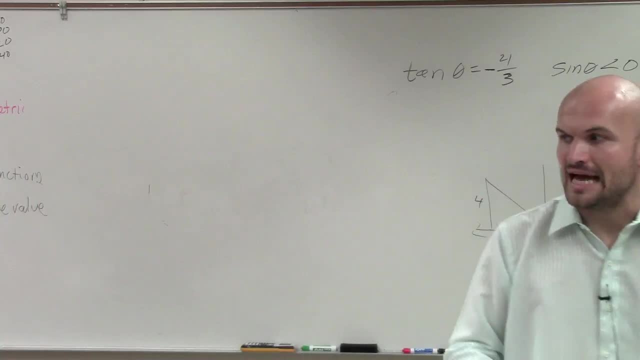 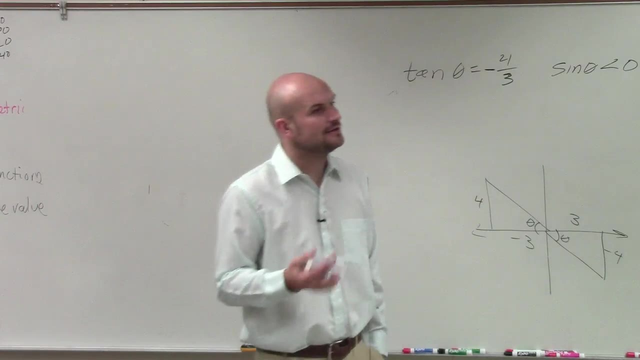 And the constraint says: sin is less than theta Or, I'm sorry, sin is less than 0. Sin of theta, I'm sorry, is less than 0.. So in what quadrants, Ahmad, What quadrants is sin less than 0?? 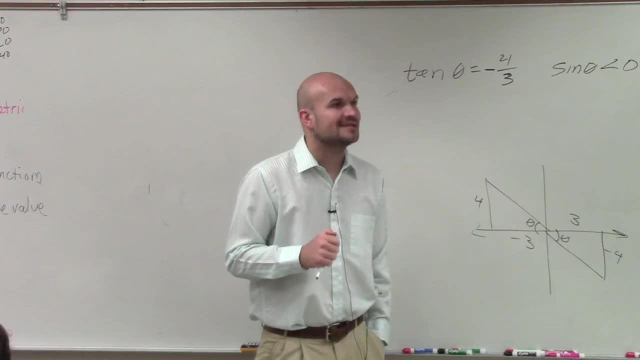 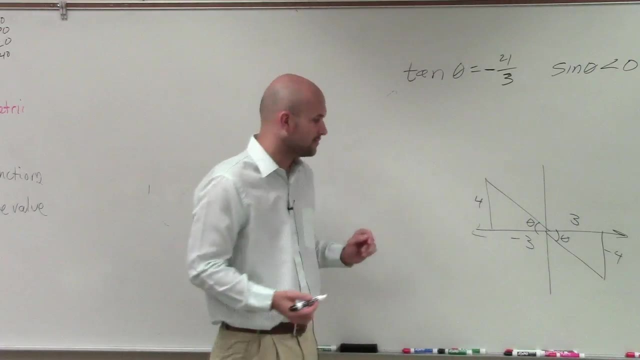 than 0.. I'm asking you, Ahmad, Exactly. Thank you, Elena. yes, Yeah, exactly. Sine is less than theta in the second or in the third and the fourth quadrant. So guess what? This triangle we're not going to use. 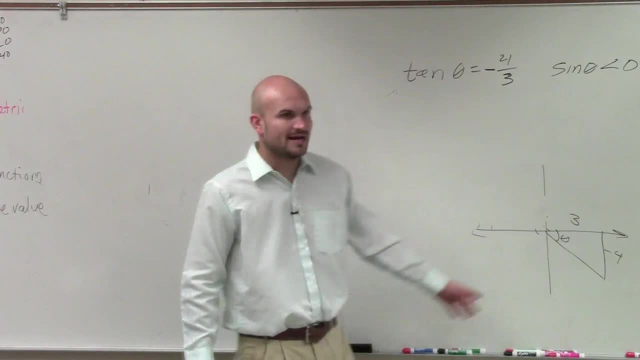 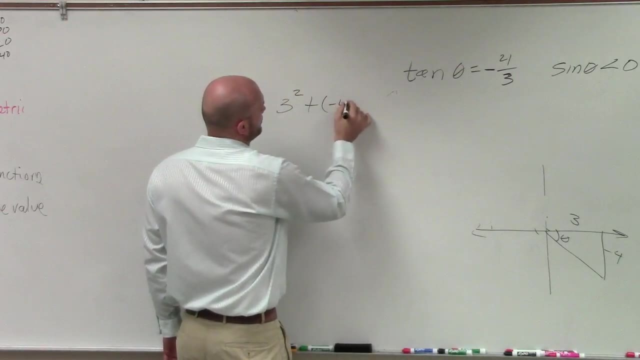 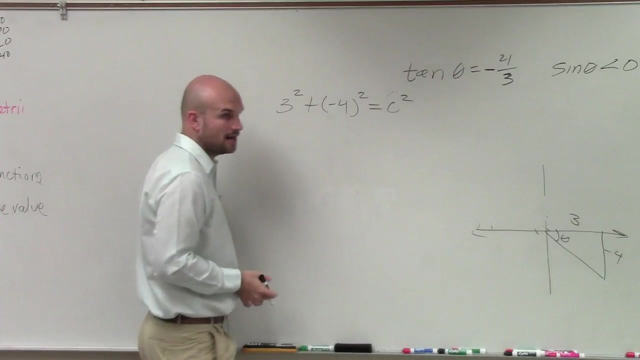 So now here's the triangle that I'm going to use, And now can I go ahead and use this to find the hypotenuse? Yes, Hopefully you guys know this is a perfect square, or a Pythagorean triple, So therefore, that's going to be 5.. 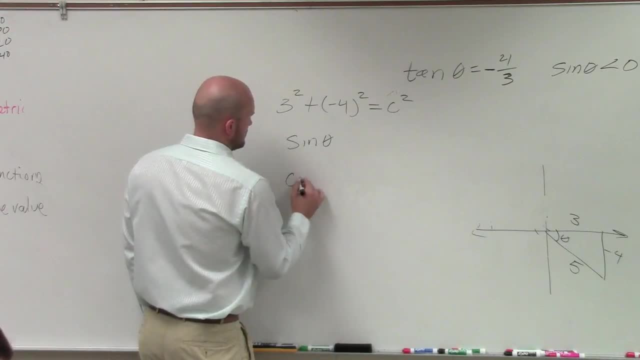 So now, if I want to find the sine of theta, cosine of theta, and we already know what the tangent of theta is. So the sine of theta is going to be opposite over hypotenuse, which is negative, 4 over 5.. 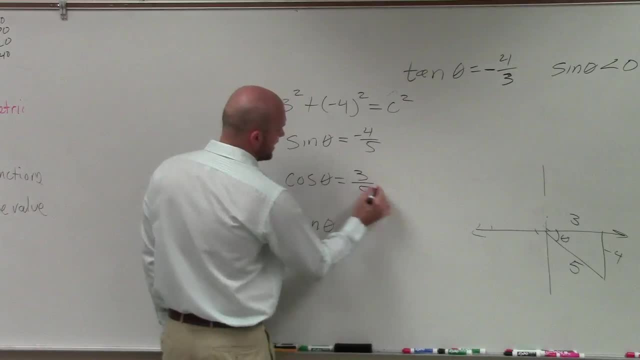 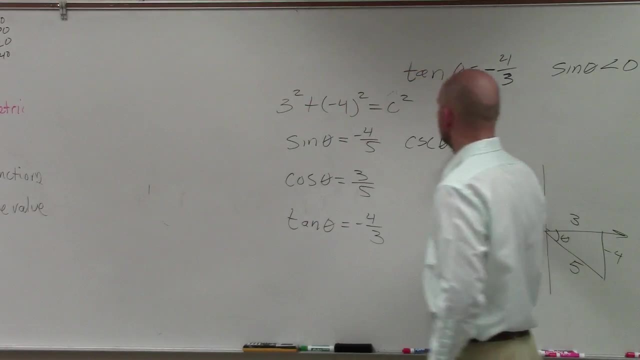 Cosine of theta, which is going to be 3 over 5.. And the tangent of theta, we already said, was equal to negative 4 over 3.. Then if I want to do the reciprocal functions, cosecant is 5 over negative 4.. 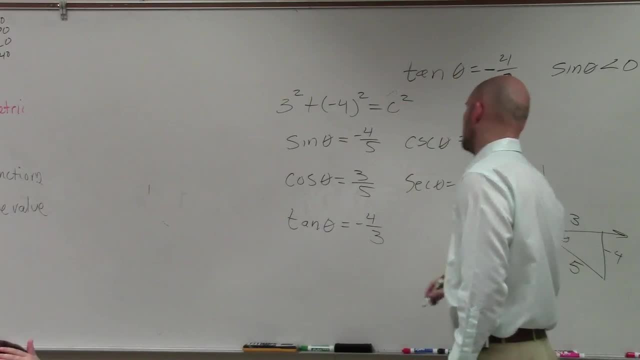 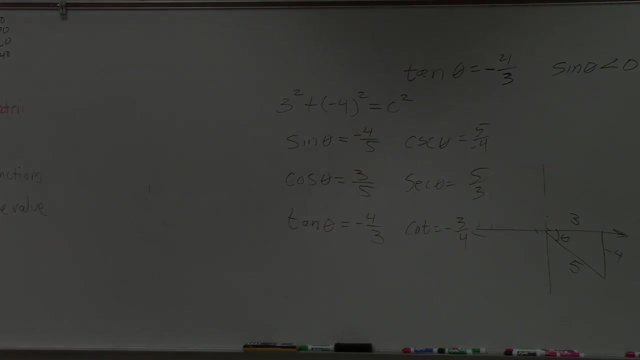 Secant of theta is 5 over 3. And the cotangent is equal to negative 3 over 4.. OK, That's it, Guys. there's way too much talk. 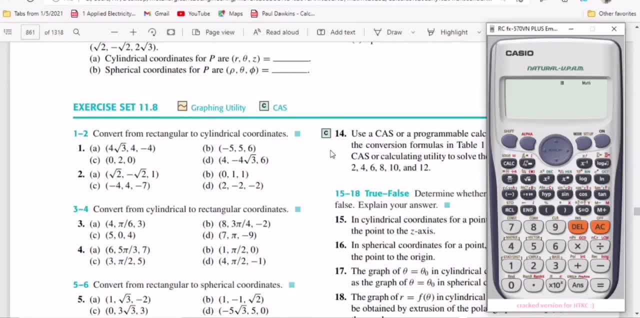 So take a calculator. So let's go there. So we're going to learn how to convert the rectangular coordinate system to the cylindrical coordinate system using a calculator. So this is my calculator, So let's get going. So let's check question number 1a. We are 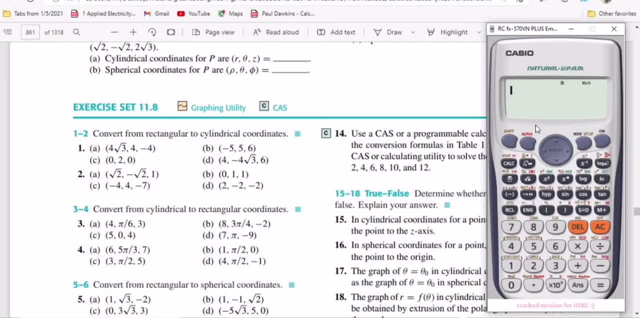 supposed to convert 2L4 with 3,, 4, negative 4 in bracket, to cylindrical coordinate. But we can do this using the calculator. Let's check how we can do it. So on your calculator we have something called a POL. So you go to shift, You press shift and go to plus. 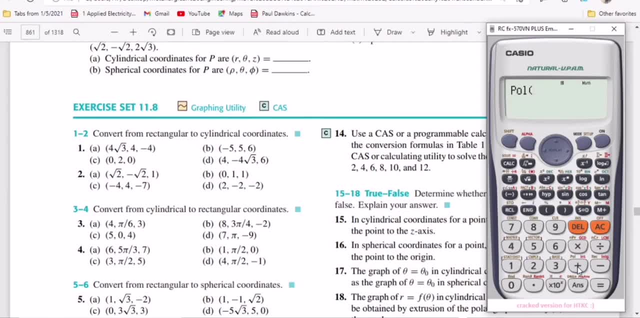 So this is the command that will change the rectangular coordinate system to cylindrical coordinate system. So what you know that with cylindrical coordinate system we have R, theta and Z. So here we are not going to include Z, So we are going to deal with. 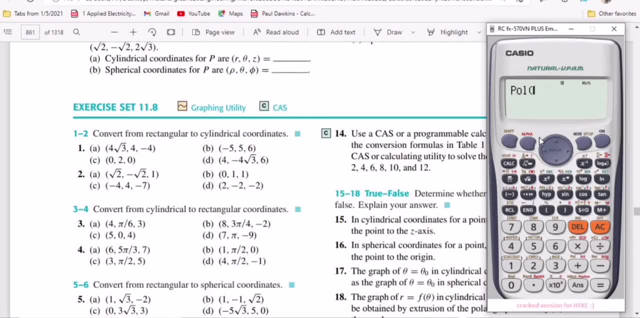 only X and Y, because Z is Z in cylindrical coordinate. So what you do now is you are going to do this, You are going to do this, You are going to do this. You are going to input the first one, which is 4 with 3.. Then you leave a space, Then you press what Shift? 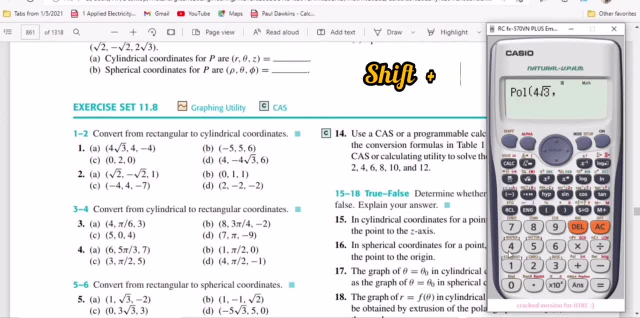 plus X, comma, right, And you put in 4.. Then you close the bracket. Note this: With the cylindrical coordinate, Z is Z, right, But the one that varies was the R and the theta. So then, when you are done, just press equal to. So with this, R is 8 and theta is 30.. 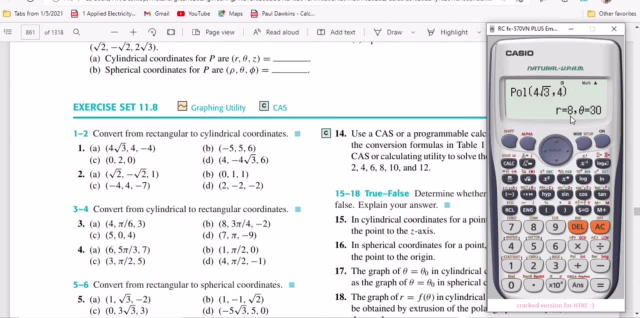 Theta can be expressed in pi. So you should note that. So you can express this in pi. So this is how we can convert the rectangular system to the cylindrical coordinate system. Let's try another one. Let's see this. Let's take